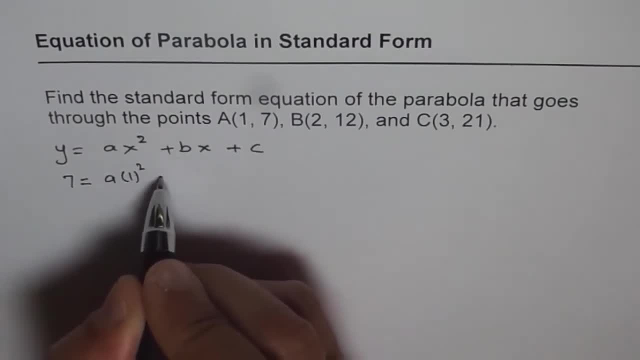 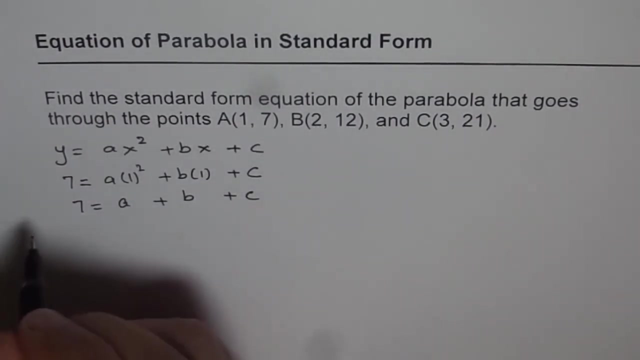 x with 1.. So we get a times 1 square plus b, times 1 plus c, And that gives us 7 equals 2 a plus b plus c. So let's call this as our equation number 1.. And here we have used the. 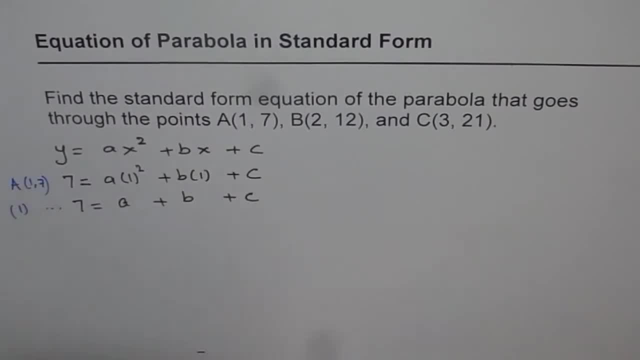 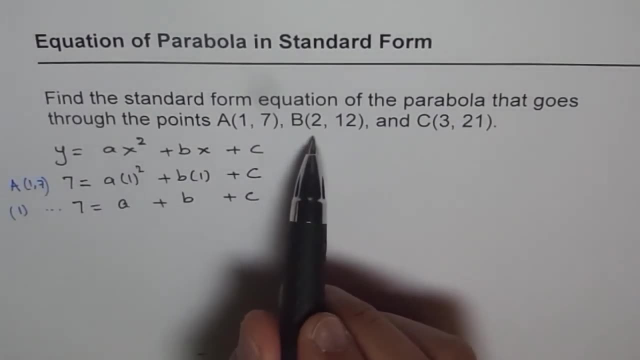 point a, which is 1, 7.. Now, similarly, what we can do is we can find the second equation by substituting b, which has a coordinate point of 2, 12.. So 12 is the y value. So we: 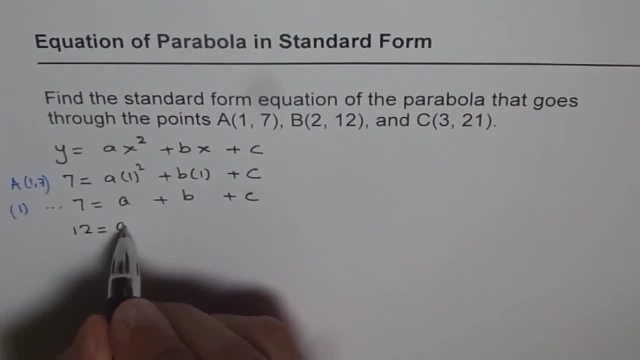 get 12 equals 2.. a times 2 square plus b times 2 plus c, So 12 is equal to 4 a plus 2, b plus c. Now we can call this as our equation number 2.. And in equation 2, we have used the point b, which 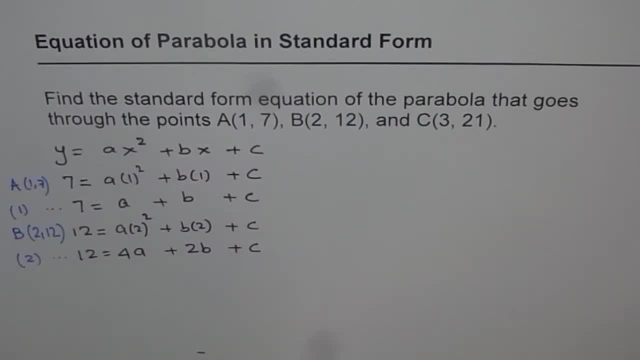 is 2, 12.. Now from these two equations what we can do is we can eliminate the coordinate C right, So from equation 2, so we can do equation 2 minus equation 1.. So if we do that, 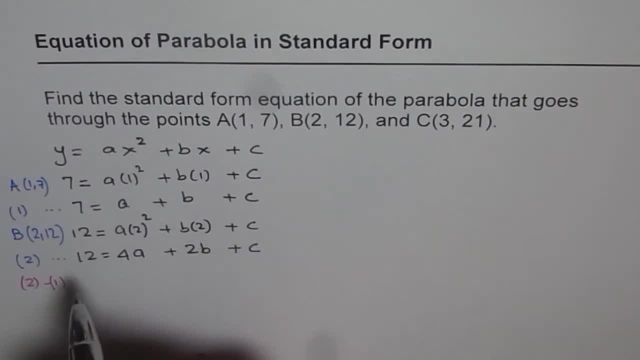 we can eliminate C from these two equations. So what we get is: 12 minus 7 is 5, equals to 4A minus A3A and 2A minus B. 2B minus B is B, so C is eliminated. Now we can also: 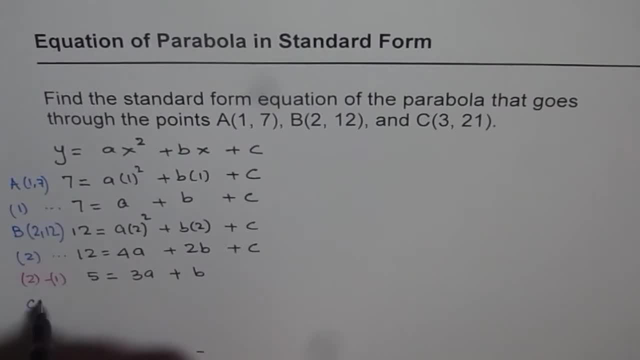 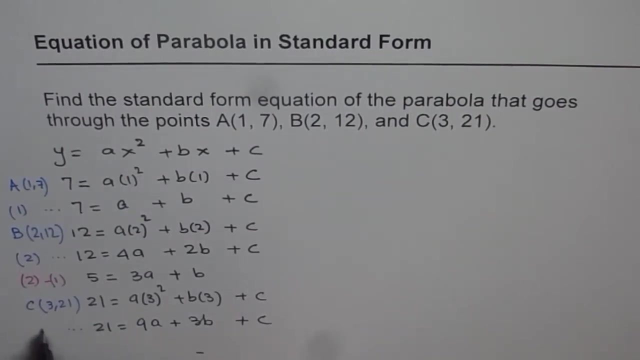 get the third equation, which is using the point C 321.. So 21 is the Y value, 21 equals to 3, 3 square is 9,. let me write 3 square first. So we get 21 equals to 9A plus 3B plus C. Let this be our equation number 3.. Well, I 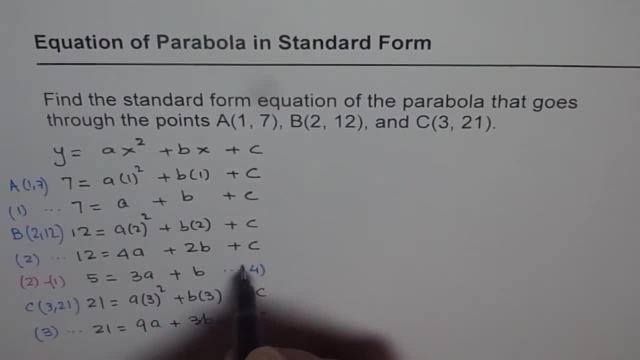 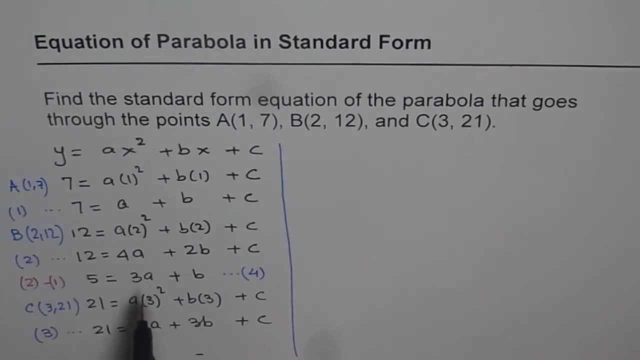 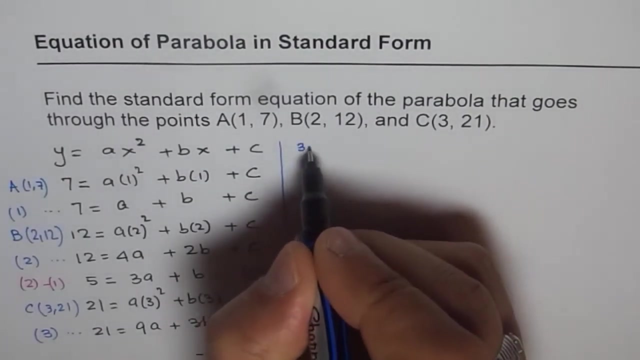 did this step here. Let me write this as equation 4, the equation derived from first and second equation. Well, we need not To eliminate C from the third equation also, so that we have equation A and B to solve for A and B. So let us use equation 1 and 3.. So we can do now equation 3 minus equation. 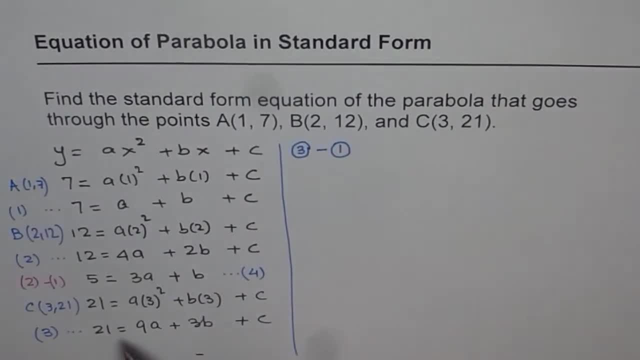 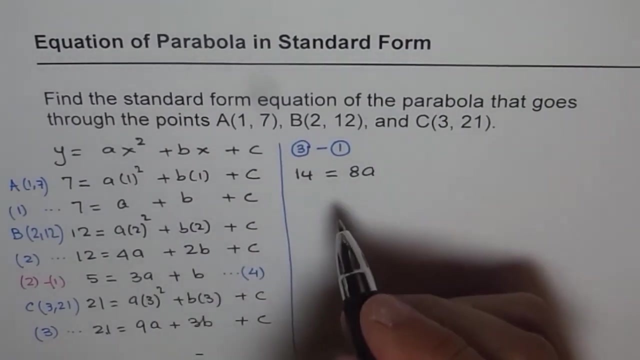 1. Then what do we get? So 21 minus 7 is 14, equals to: 9 minus 1 is 8A, And 3 minus B is 2B. We get 2B. Now this can be simplified. We can divide by 7,. rather. 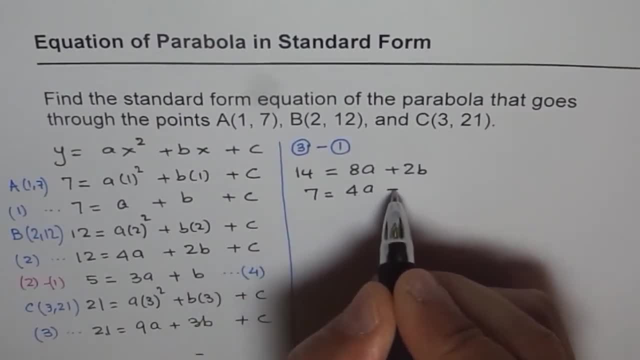 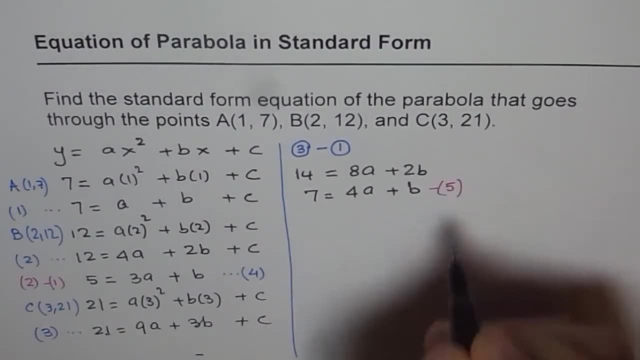 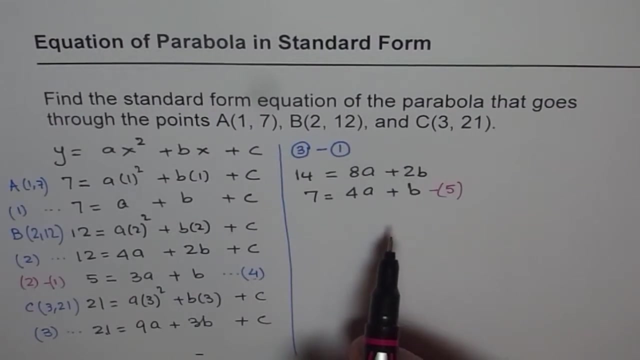 2, to get 7 equals to 4A plus B. Now let me call this as equation number 5 for us. Now we have equation 4 and 5, which have only 2 variables, which are A and B. Now, if I do, 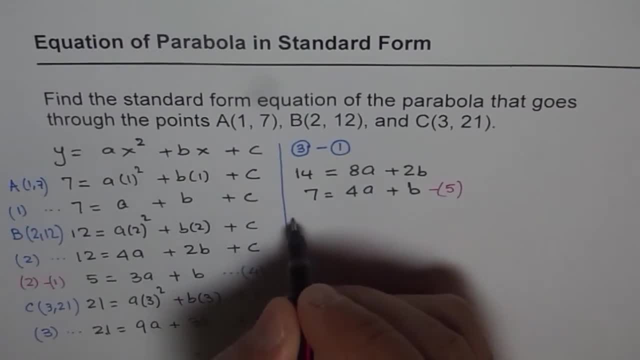 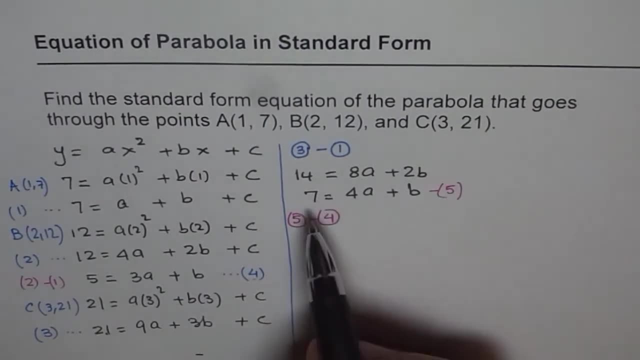 equation 5, I can minus 4, I can eliminate b, So we'll do equation 5 minus equation 4.. 7 minus 5 is 2.. 4 minus 3 is a, So we get a as equals to 2.. Now, once we get a equals to 2, we can write this equation: 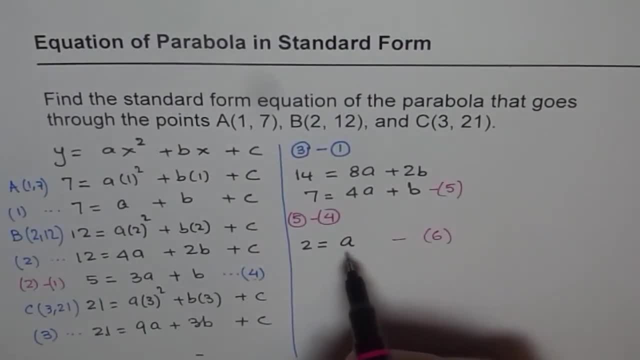 as equation 6.. We can eliminate or we can substitute a in one of our equations with two variables and find b. So let me substitute a equals to 2 from equation 6 in 5.. So let's go backwards to find the values of b and c. So we get 7 equals to 4 times 2 plus b, or 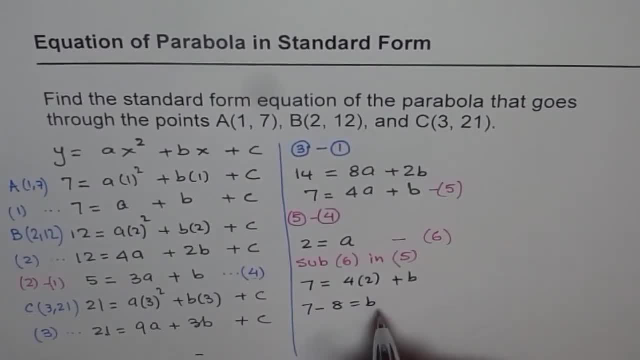 7 minus 8 equals to b, which gives us value of minus 1 for b. So we get equation 7, where b is equals to minus 1.. Now we can use one of our original equations, Let us say equation 1.. So we'll. 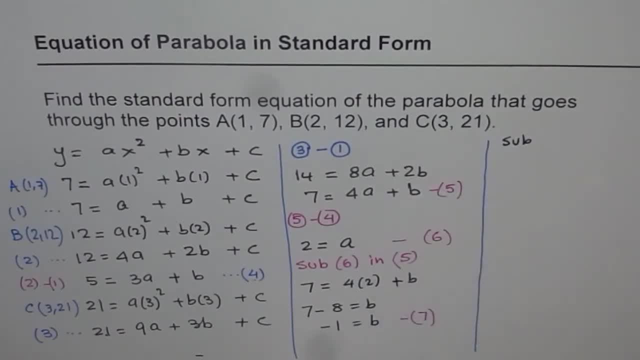 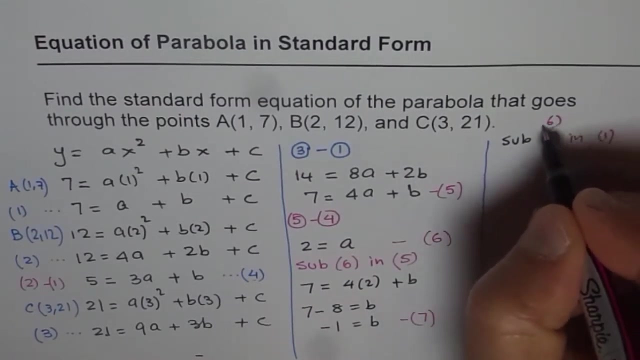 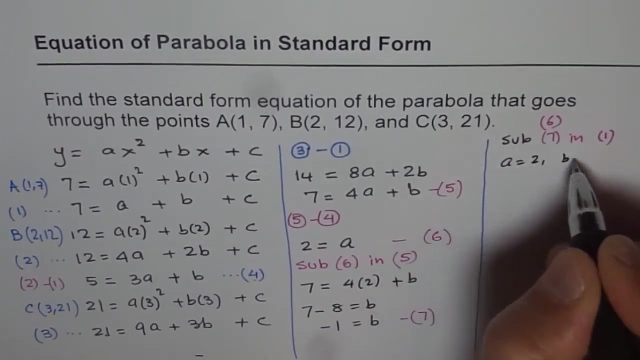 sub equation 7 in equation 1.. So that way we'll sub the values of a and b Also 6.. So a, we know, is equals to 2. B is equals to minus 1, and we have substituting these in equation number 1. So we have 7 equals. 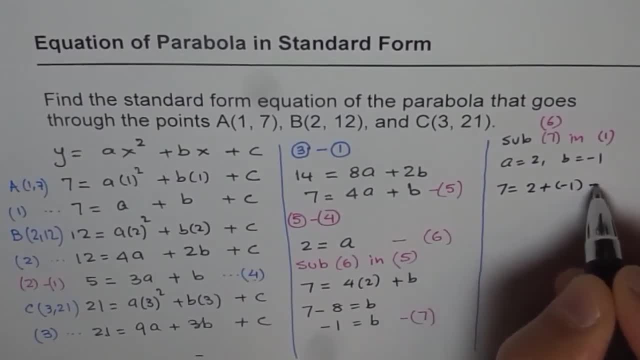 to 2 plus minus 1 plus c. So that is 7 equals to 2 minus 1 is 1 plus c, And we get 7 minus equals to c, which is equal to 6. with that we get our equation right. so from. 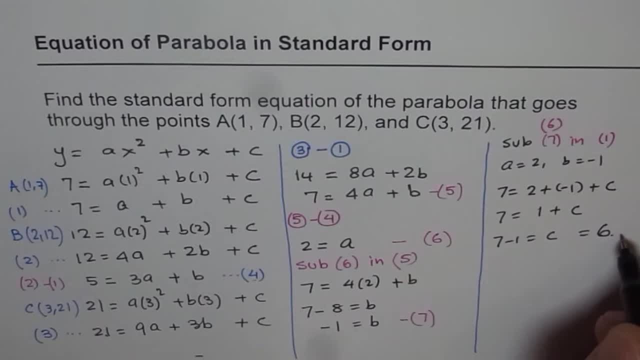 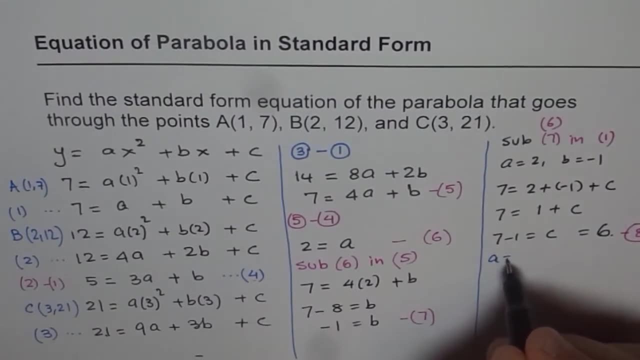 the starting equation this. let me call this as equation number 8. so now we know that a is equals to 2, B equals to minus 1 and C equals to 6. that gives our equation, which is: y equals to 2x square minus X plus 6. so that is a solution for. 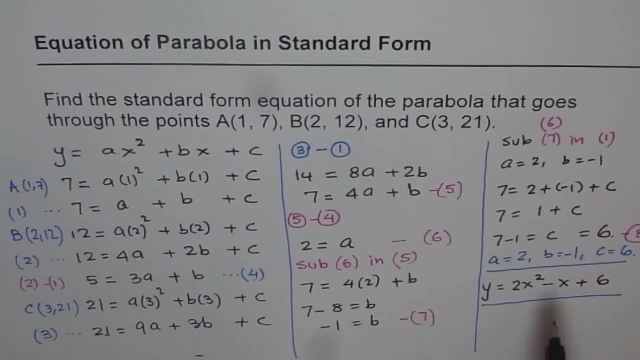 this problem. you can always verify, once you get your standard form equation, that these points really lie. on that you can substitute 3 for X and figure out if you really get 21 for Y. that's the way to check it. now let's review how we did it. 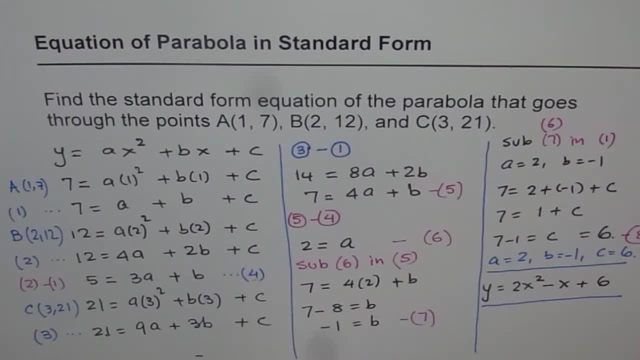 so we've given three points: a, B and C. with these three points we get three different equations with three unknowns. now, whenever you have three equations with three unknowns, it is possible to find the values- values of unknown- by following systematically method of elimination and substitution. so this: 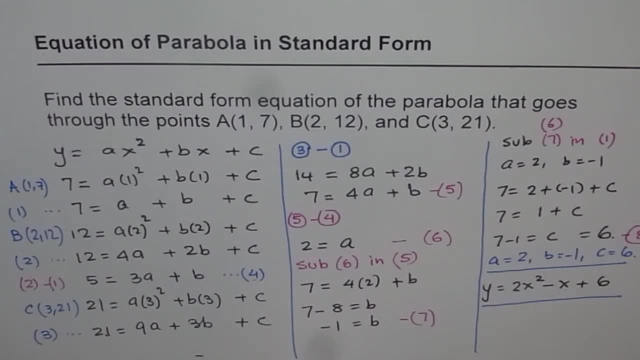 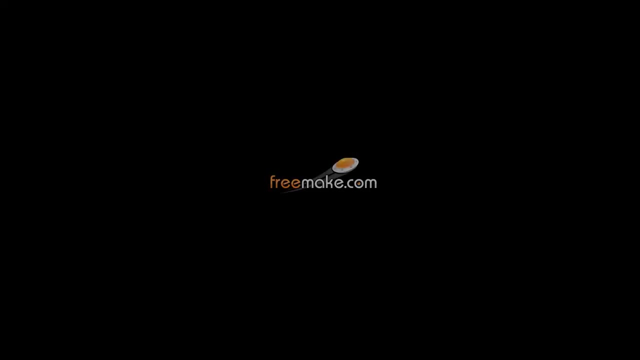 example actually illustrates the method, and once you follow this method, as shown here, you can always get your equation. so we will do two more examples, which will be slightly more complicated than this, and then move on further. thank you and all the best.